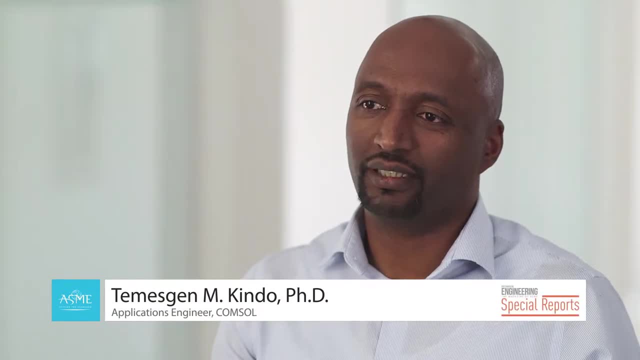 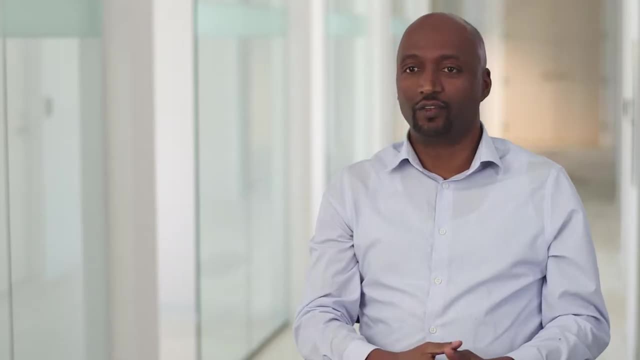 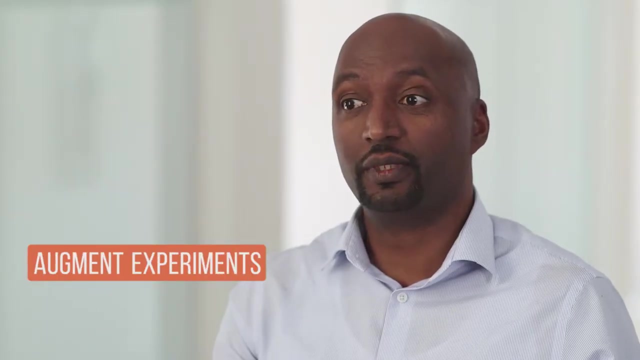 Simulation software is growing more important in the design of products, especially in the biomedical industry, because of the following three reasons: One is the need to handle multi-physics problems. The next is to replace or augment costly or difficult experiments. And finally, the need to solve novel problems. 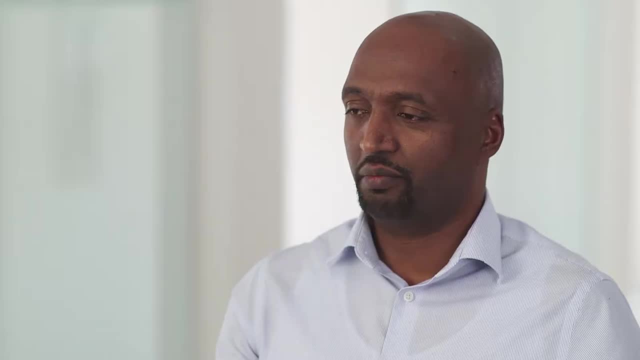 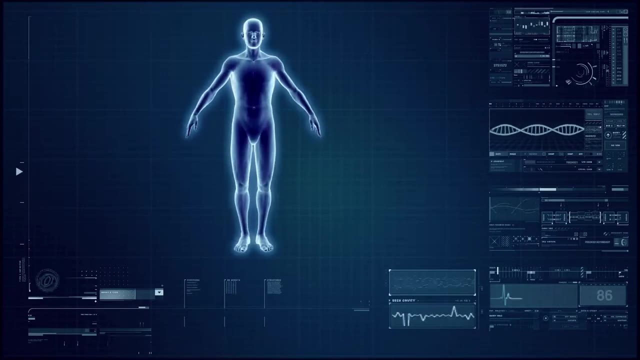 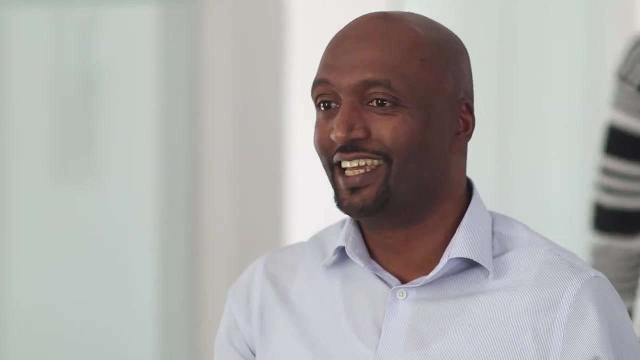 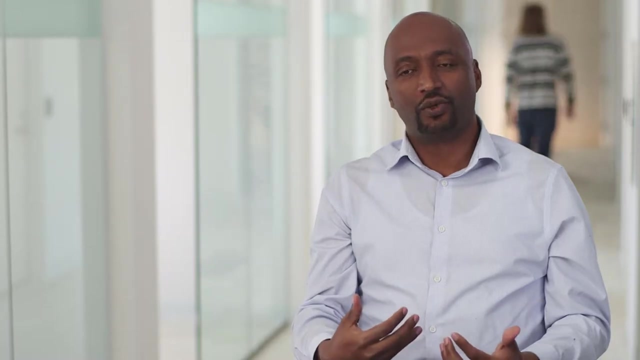 What we mean by solving novel problems is in biomedical engineering, for example. it's a combination of solving for physics and solving for engineering. How do you model healing? Engineers are used to just modeling damage, for example, but then bodies heal. How do you model that As a biomedical engineer or as a practitioner? you might have to bring in new equations to handle this. And do you have tools to kind of take that and couple it with the existing physics? 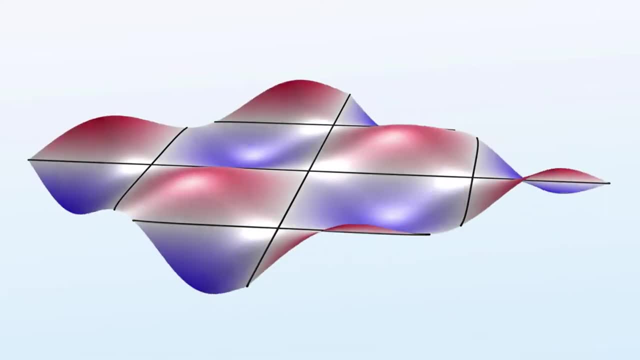 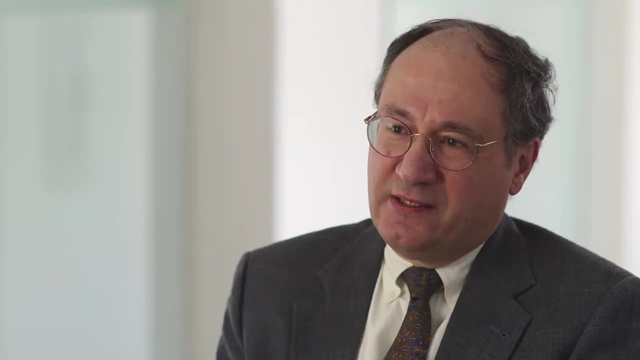 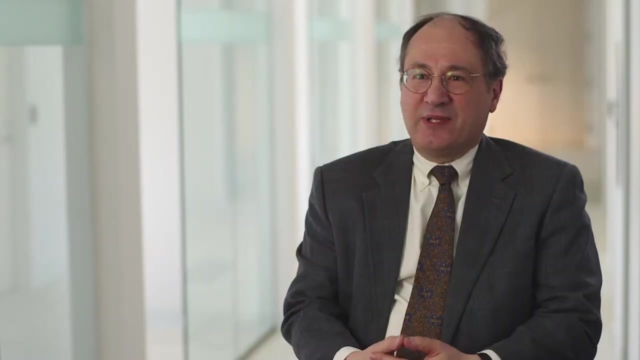 Well, simulation has two functions really. One is to help the design effort, set parameters up For optimizing a design and understanding what's going on. And when I deal with development engineers that are in the lab, it also enables them to investigate what's going on in places. they can't go. 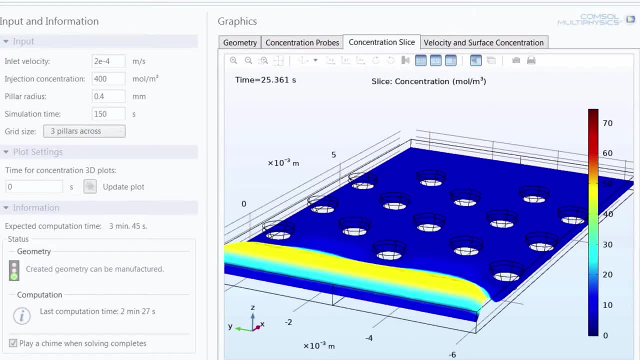 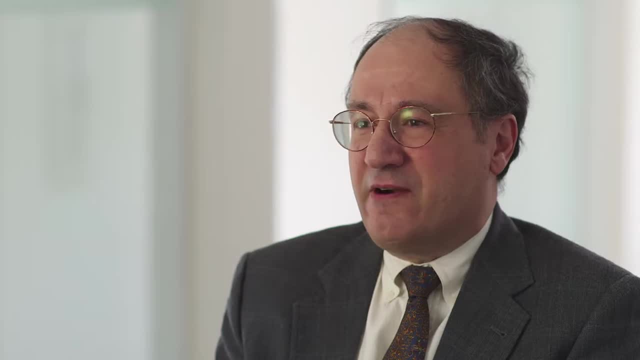 A lot of what comes out is animations of what's going on with flow or heat or other physical phenomena, and they can use that to present to their management. It's a very clear way of showing what's going on and it's a really valuable tool. 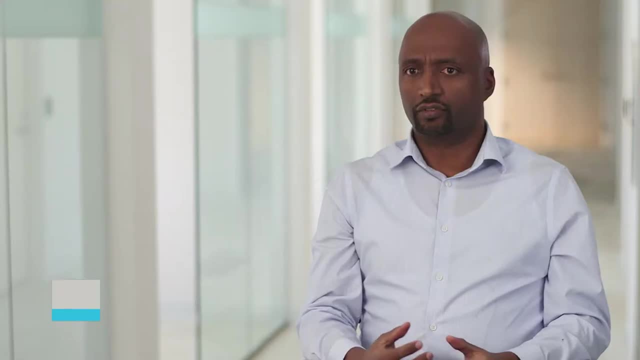 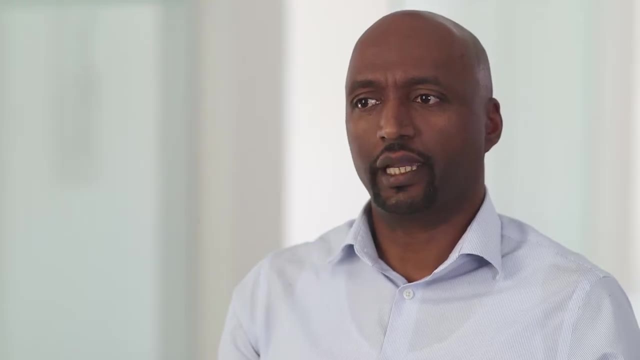 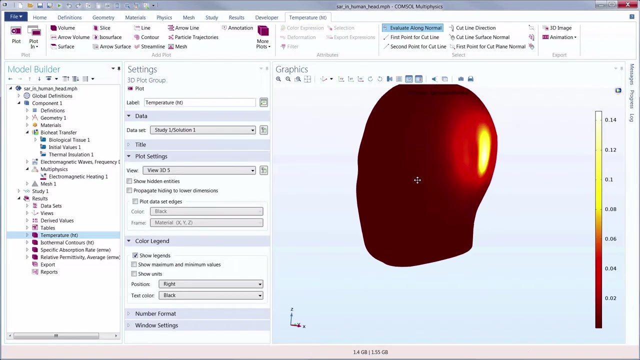 Simulation software is a megacommunications machine. It can between different engineers, different specializations within engineering, easier, as well as make it possible to effectively communicate between engineers and non-engineers. Simulation makes communication with non-engineers more clear. Communication with non-engineers is essential. 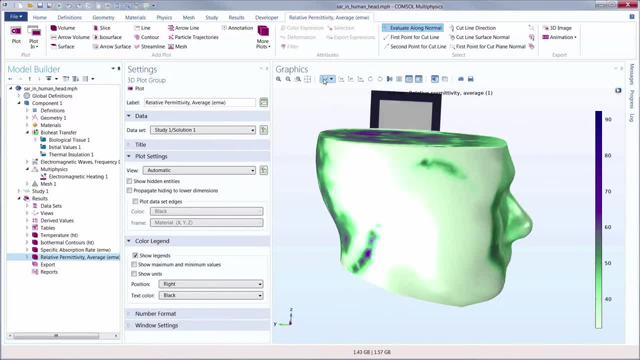 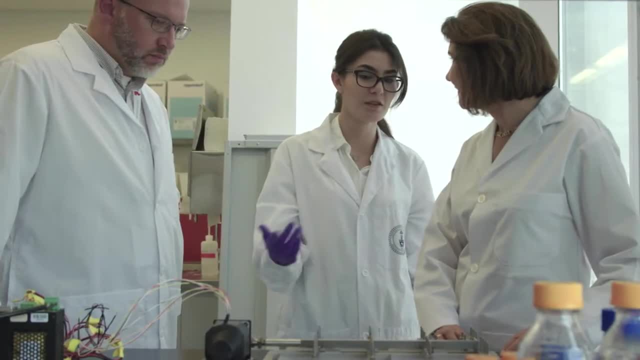 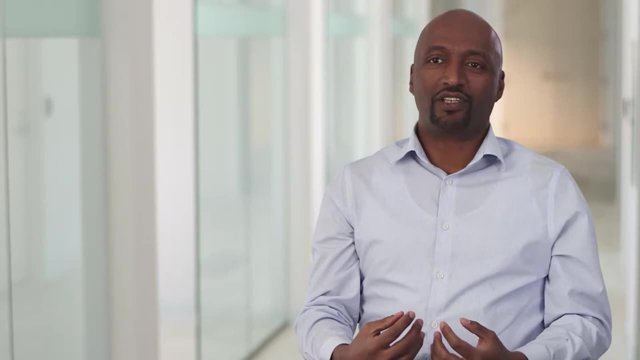 And the role where we come in is the initial prototyping and design. That involves having to understand the basic technology from the scientist or clinician that initially develops it and then develop that into something that's going to bridge over to manufacturing. Engineers might be interested in looking at physics quantities whereas, say, a clinical.